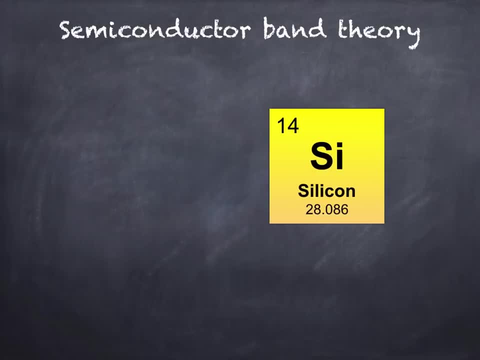 So first of all we're going to look at the element silicon, although other semiconducting materials are available. Silicon has the symbol Si and an atomic number of 14.. This means that silicon atoms contain 14 electrons, Two in the first shell, eight in the next, then 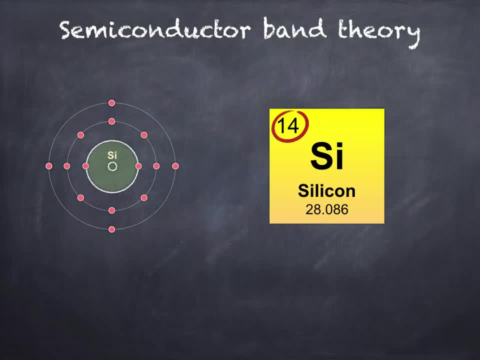 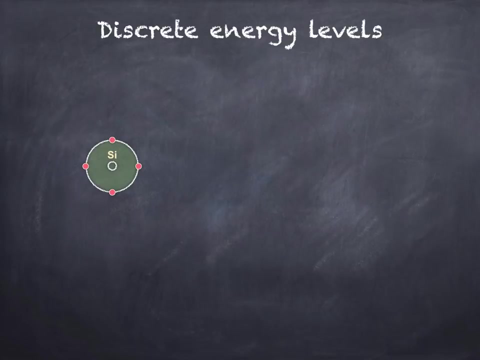 four in the outer shell. We refer to these outer electrons as valence electrons. These are the electrons which can form chemical bonds. Now we'll simplify a model of the silicon atom to show only the four outer valence electrons which take part in bonding. In individual atoms, the electrons can only occupy discrete. 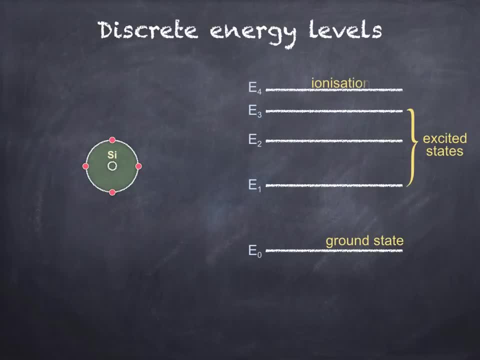 energy levels, The production of line emission spectra and line recycling and storage of an electron and the processing of it during the process. line absorption spectra can be explained in terms of the electrons moving to different energy levels and either emitting or absorbing a photon, although that's covered in another lesson. 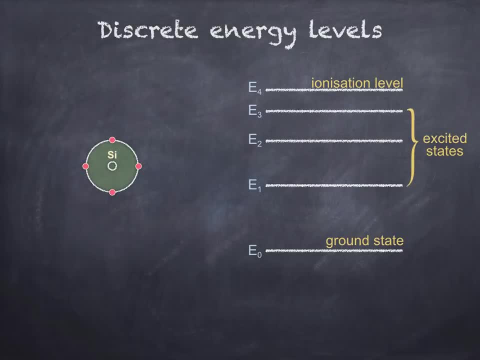 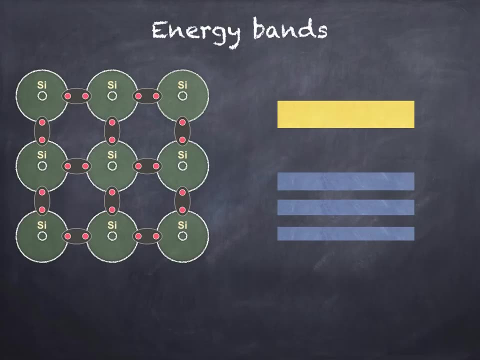 When a large number of atoms come together to form a solid, the energy levels become reorganised into bands. as the atoms interact, Each energy band actually consists of many, many closely spaced energy levels. You can see from the diagram on the left that all four of the silicon atoms' 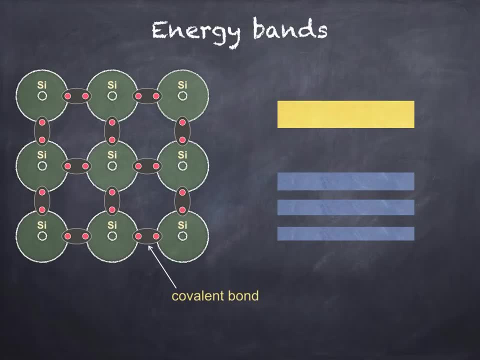 outer electrons form covalent bonds with the neighbouring atoms, Now out of interest. the diagram on the left shows what's known as the semiconductor bonding model. At zero Kelvin, all of the outer electrons are bonded. The diagram on the right shows the energy band model. 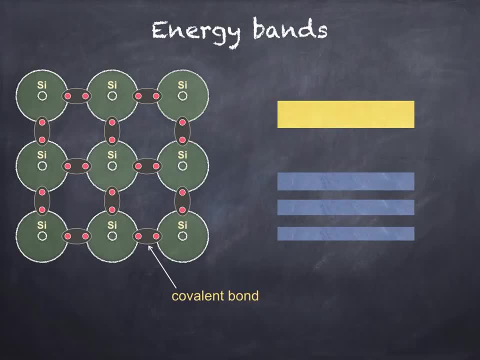 In order to explain the electrical properties of semiconductors, we only need to consider two energy bands: the valence band and the conduction band. These are separated by a band gap, which we'll discuss later. What I've not mentioned yet is that this is an undoped semiconductor of pure silicon. 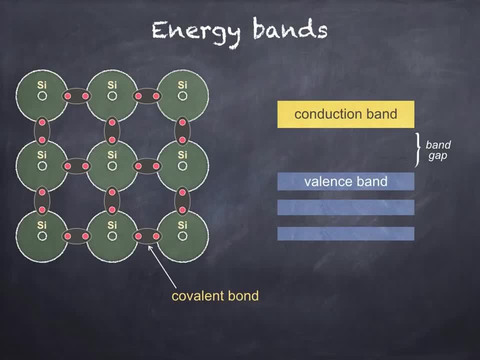 what we call an intrinsic semiconductor. As I said before, at zero Kelvin all the outer electrons are bonded. Let's look at what happens when we add some heat. So an electron has gained enough energy to break the covalent bond and is now free to. 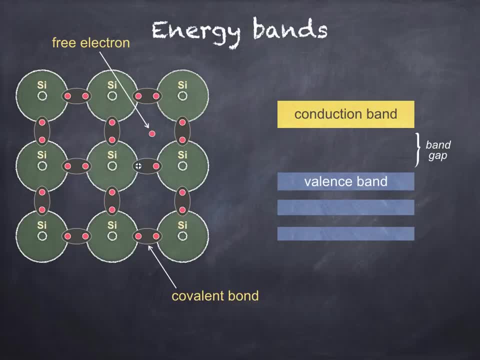 take part in conduction, meaning that the resistance of the material is reduced. The absence of the negatively charged electron in this position leaves behind a net positive charge, which we call a hole In terms of energy bands, the electron which was initially 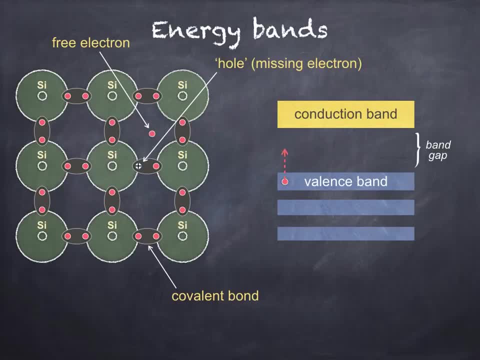 in the valence band jumps to the conduction band, leaving behind a hole in the valence band. The band gap, or energy gap, is just the energy required for the electron to break the covalent bond and jump into the conduction band. As the semiconductor is further heated, more covalent. 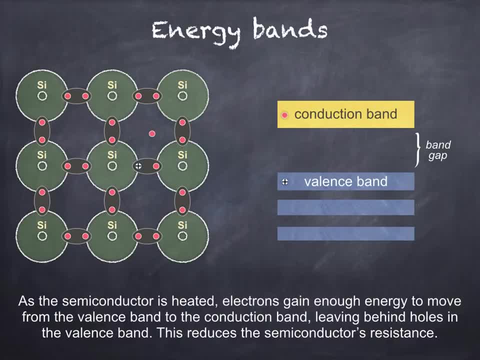 bonds are broken, So the electron is now free to take part in conduction, meaning that the electron is broken, resulting in more electrons jumping to the conduction band with more positive holes created in the valence band, So as the temperature of a semiconductor increases, its resistance. 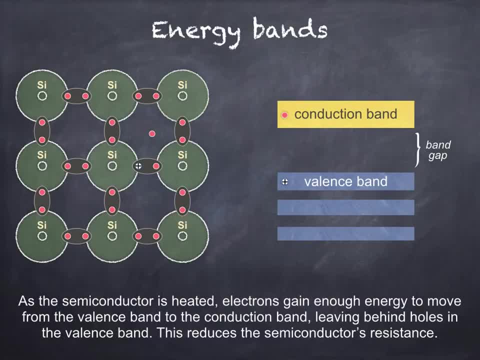 decreases due to the motion of the electrons in the conduction band and holes in the valence band. If we look at the diagram on the left, we can see that electrons from neighbouring atoms can move to fill a hole, leaving behind a hole in their previous position. 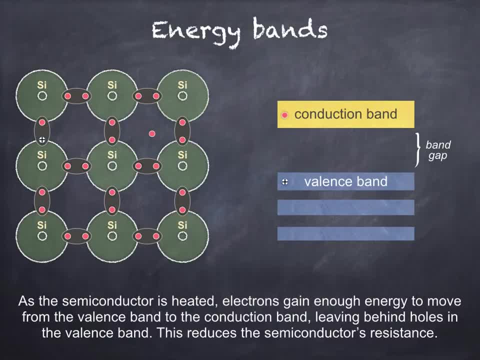 Although strictly, this was caused by the motion of negative electrons from left to right, we can also describe it as the motion of positive holes from right to left. Next we'll look at energy bands in a little more detail. As I said before, we only need to consider: 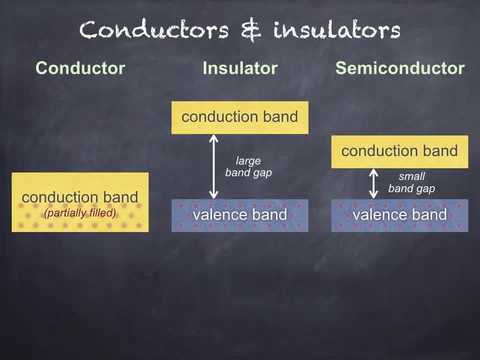 the valence band and the conduction band in order to explain the electrical properties of semiconductors and, for that matter, conductors and insulators. Remember, then, that in order for a material to conduct, it must have electrons which are free to move within its conduction band. 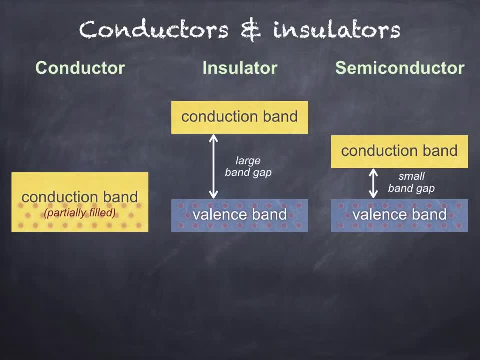 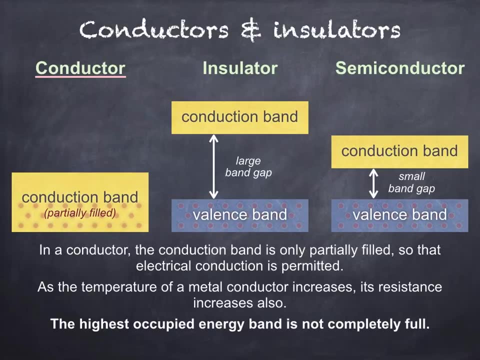 or holes in its valence band. In a conductor, conduction can actually be explained by considering only the conduction band. The conduction band is only partially filled, so electrical conduction is permitted, Unlike a semiconductor, though increasing the temperature of a metal conductor will. 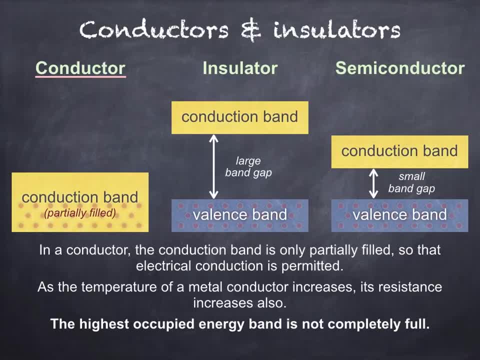 actually cause its resistance to increase. This is because the number of electrons within the conduction band increases so much that they have less freedom of movement. Remember that in a conductor, the highest occupied energy band, the conduction band, is not completely full. 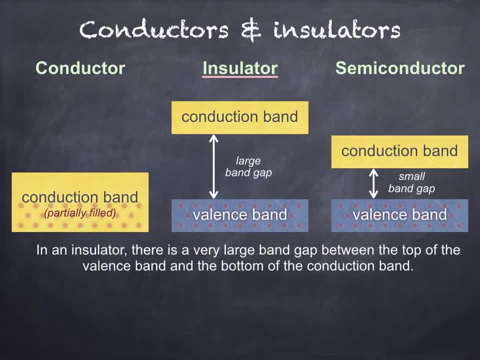 With a new valence band- the escaping valence is usually другие. energy band 1: The persuasion band is completely overfilled and the conduction band is completely empty. 2: The patrons of residences are just enough so that the induction band can move at all times. so only electrons can move. Small valves may not turn THROUGH a remote or auto-emmayınable use of the conduction band for a Brown strategy. At zero kelvin the valence band is completely full and the conduction band is completely empty. At higher temperatures electrons don't normally gain enough energy to jump from the valence band to the conduction band. So with no electrons in the conduction band conduction isn't possible. For an insulator then the highest occupied energy band, the valence band, is full. 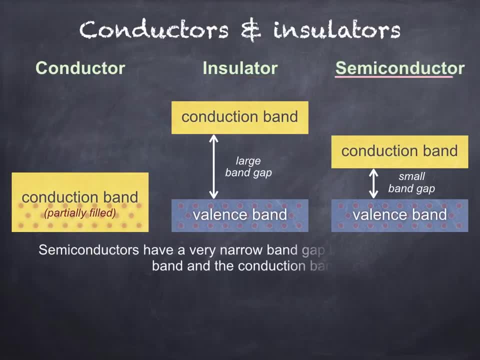 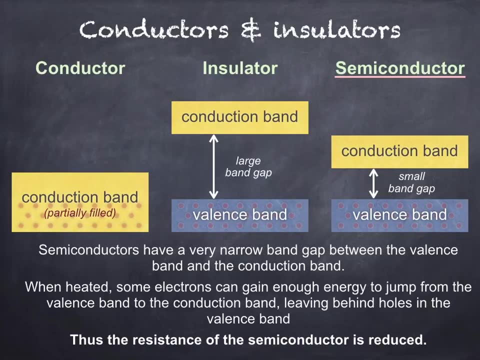 For an insulator, then the highest occupied energy band, the valence band, is full. Finally, semiconductors have a very narrow band gap between the valence band and the conduction band, Like insulators. at zero Kelvin, the valence band is completely full and the conduction band is completely empty. 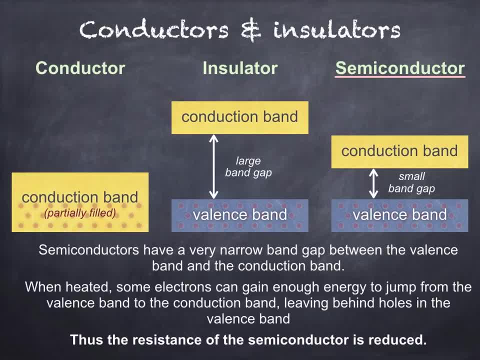 But since the band gap is so small, as temperature rises some electrons can gain enough energy to jump from the valence band to the conduction band, leaving behind holes in the valence band As temperature increases, then the resistance of the semiconductor is reduced. 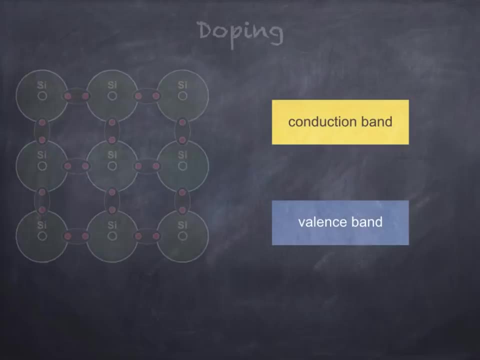 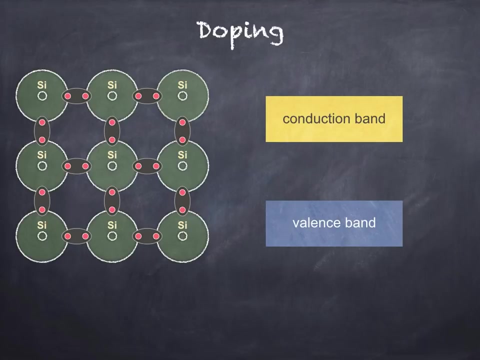 Next on the agenda is doping. Here on the left we see the bonding model of an intrinsic semiconductor, silicon. again With the addition of impurity atoms during the manufacture of the semiconductor, we can reduce its resistance. This is done in one of two ways. 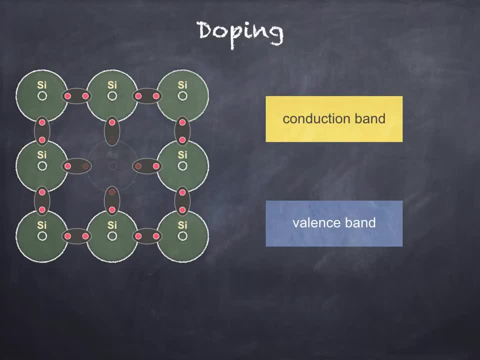 By doping with a group 5 impurity atom such as arsenic, as shown here, we end up with an extra electron. The energy level of this fifth electron is within the band gap, just below the conduction band. The energy levels associated with the extra electrons are known as donor levels. 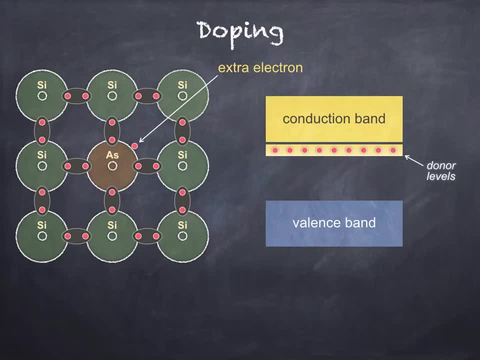 Even at room temperature, most of these electrons will gain enough energy to jump into the conduction band, thus reducing the resistance of the semiconductor. We call this an n-type semiconductor, since the majority of conduction is due to the negative electrons within the conduction band. 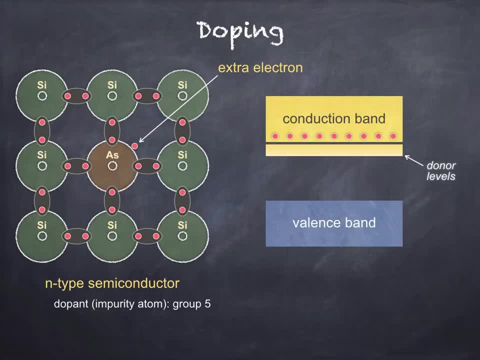 Remember that we previously discussed the heating of an intrinsic semiconductor. For each electron which jumped from the valence band to the conduction band, there was one hole in the conduction band. There was one hole left behind in the valence band. This meant that in an intrinsic semiconductor, electrons and holes exist in equal number.